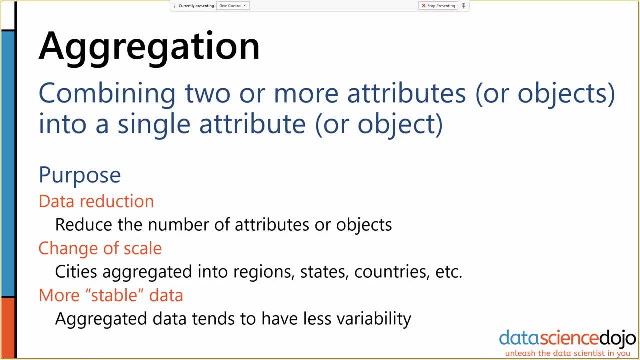 you know, 10 or 15 different sessions for that user. So the reason why we do this is exactly that, If we want to average user times, for instance, we're changing our scale. We want to aggregate cities into regions, states or countries. We 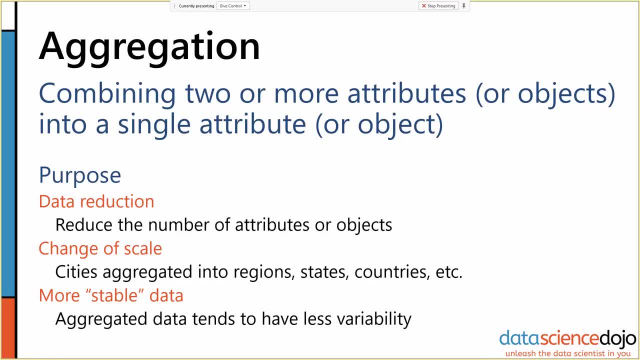 want to aggregate dwell times across sessions or across pages, And one of the big advantages of aggregation- particularly averaging- is that aggregated data tends to have less variability. It's a way of reducing the number of data objects that are aggregated, And so we want to aggregate. 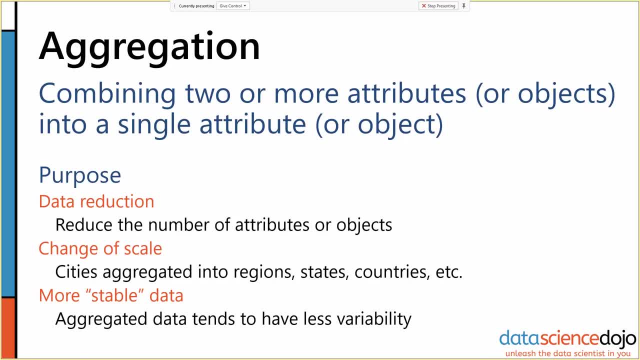 data in a way that's more consistent with our data. So we're going to do this by reducing the effect of noise. Well, it's a way of reducing the effect of random noise. If you've got human labeling errors, then you've got human labeling errors. If you've got, you know, if you've got. 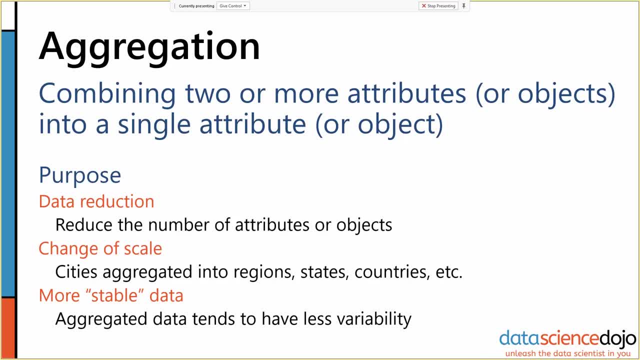 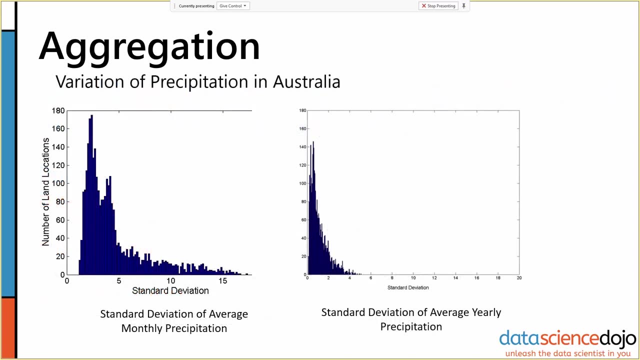 sampling procedure errors. you have sampling procedure errors, But if you've got random errors- say you're you know random noise- then aggregated data will very much tend to reduce that. So as an example of that- and I really like this next page for this- these two are graphs. 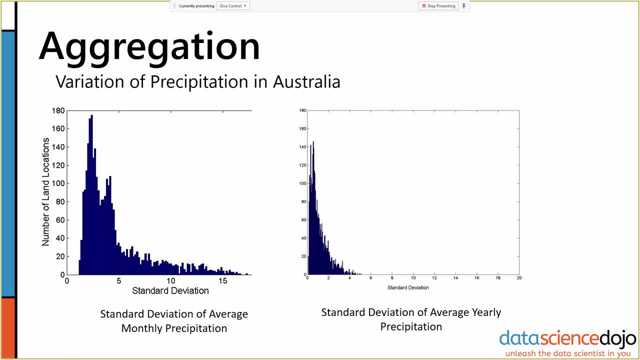 of precipitation in Australia, So every. so. these are histograms, So the height of each block is the number of locations where precipitation was measured, which had, in this case, a standard deviation of between zero of the x value when we measured it on a monthly basis. 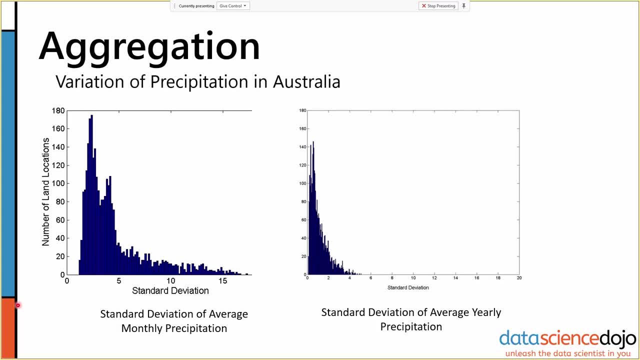 So we're measuring the average monthly precipitation and measuring the standard deviation of that monthly precipitation at you know, 500 different land locations in Australia. When we do that on a monthly basis, we get this very wide spread of standard deviations. Some places are very consistent in their rainfall, Other, you know, there's kind of these two peaks. 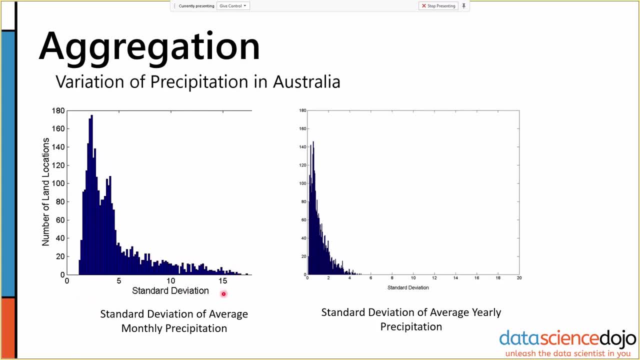 and then you have this long tail of places that are just all over the place in terms of the variability in precipitation. On the other hand, if we take those exact same land locations and instead find the average yearly precipitation, the very, very standard deviation of that,